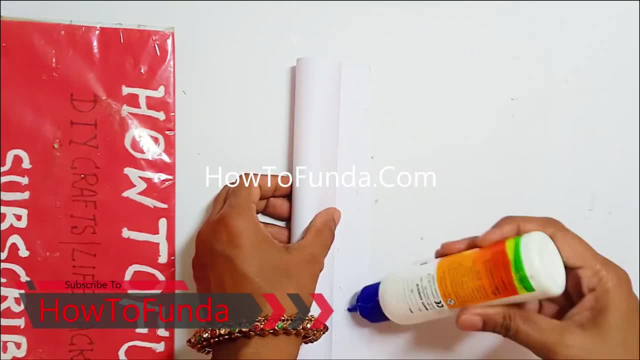 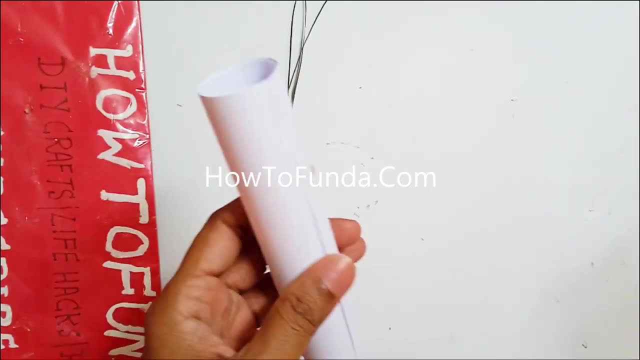 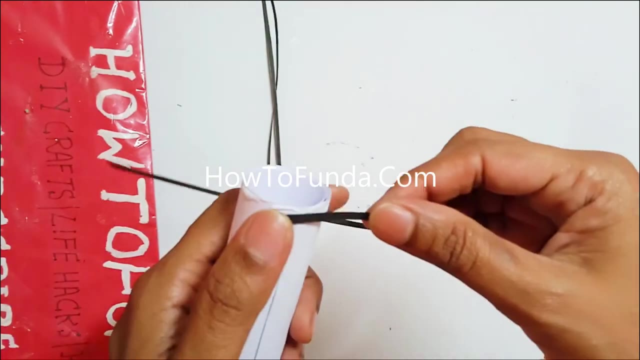 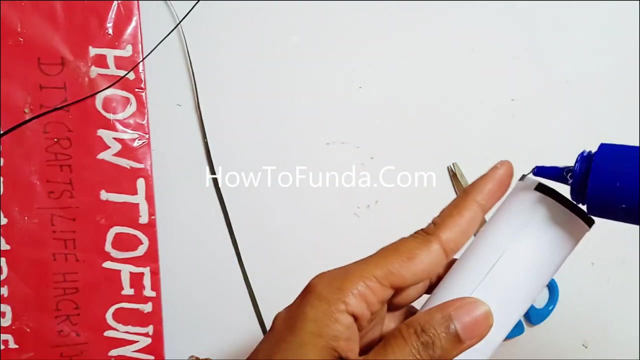 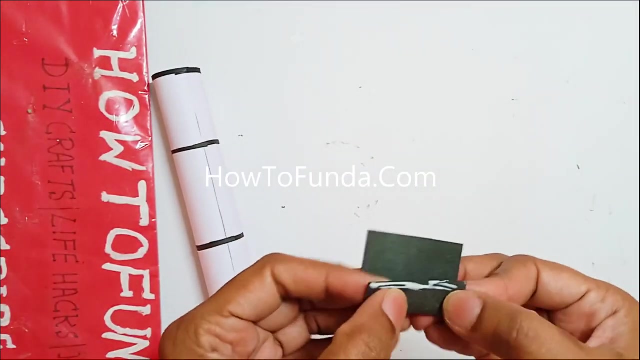 Thank you for watching. I'm inspired by thirst. I'm inspired by thirst. I'm inspired by worth. I desire your worst, So you can just hide while I work. I ain't tired you. first I'll write a second, third verse. 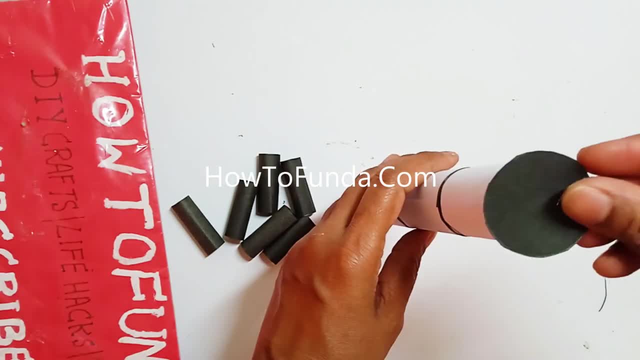 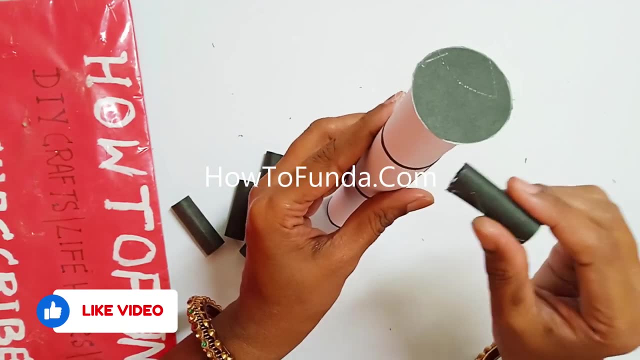 About the lies you go disperse. You never did s***. I know it hurts, But something deep inside won't let me quit. I swear that I'm inspired by all this s***. Tell me that I can and I won't. 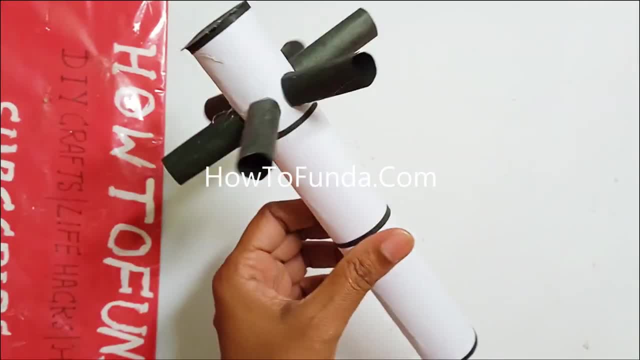 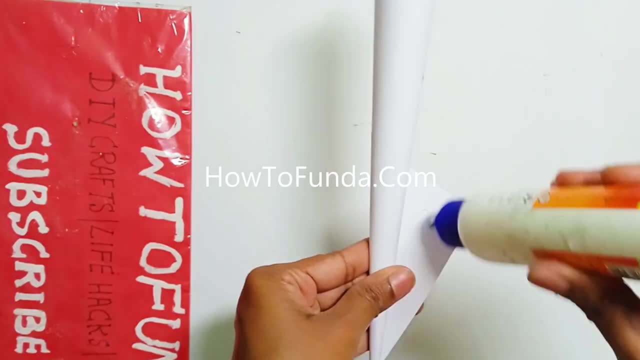 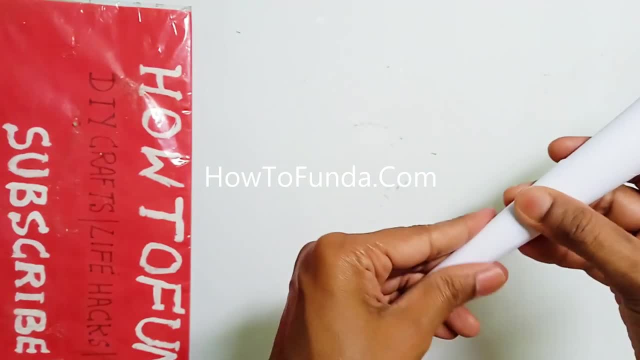 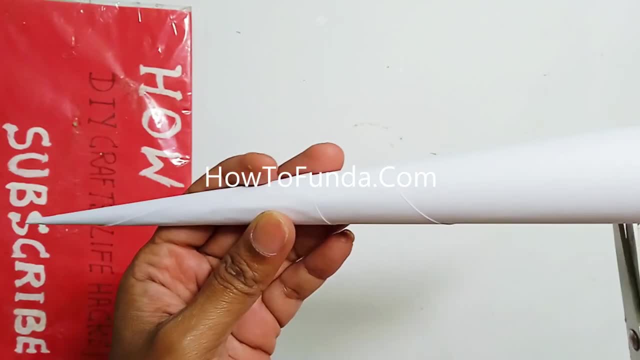 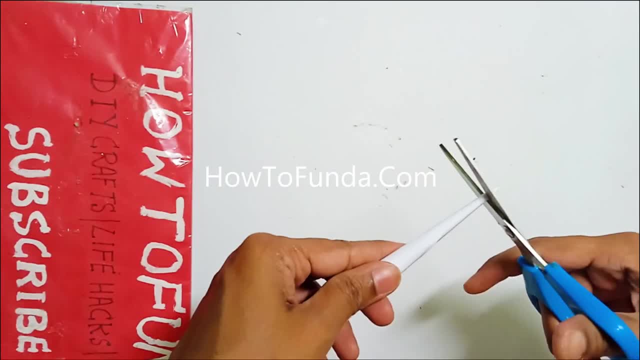 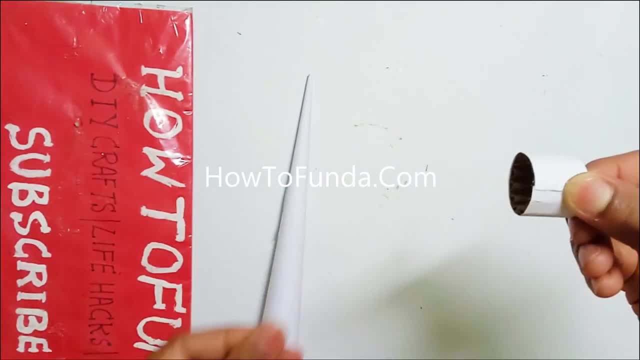 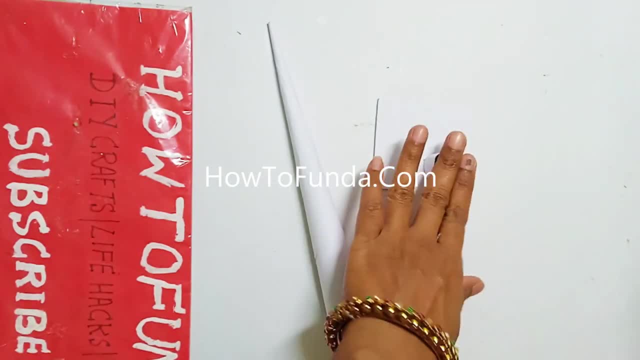 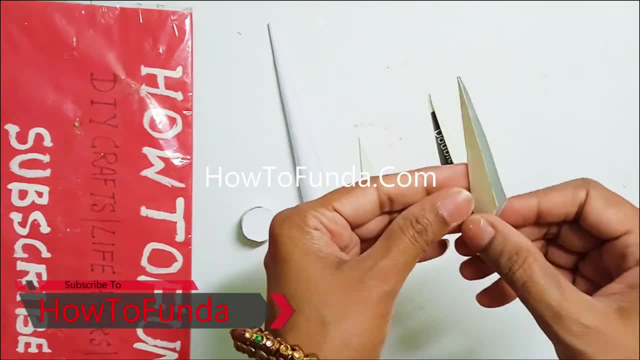 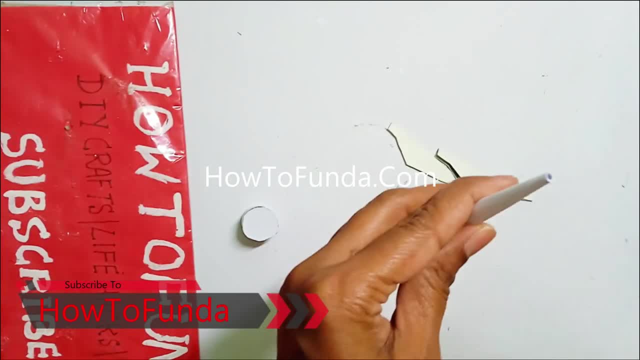 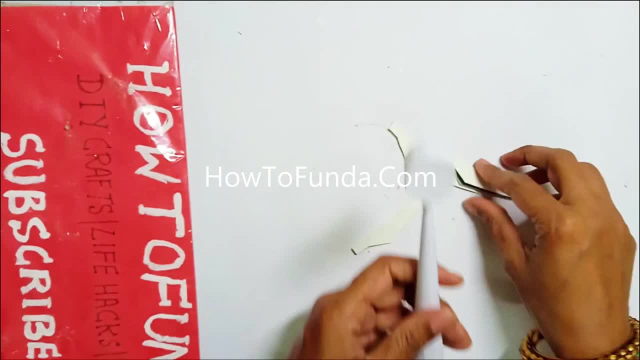 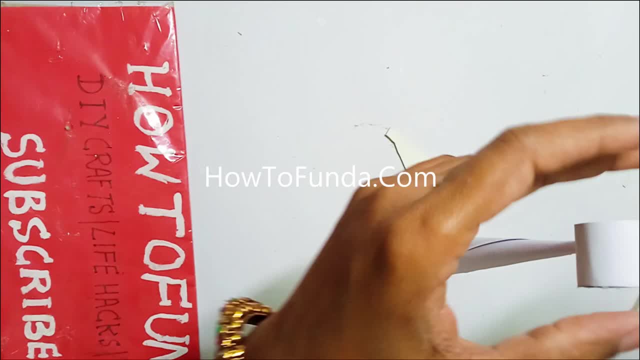 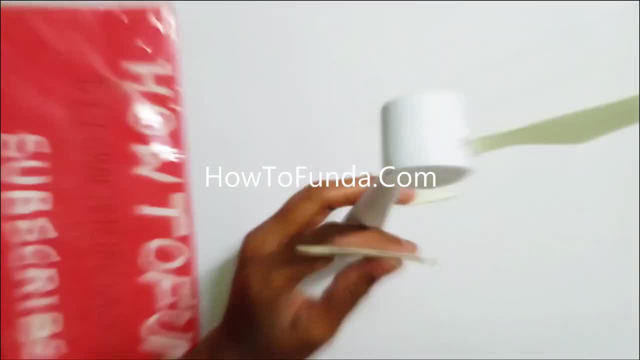 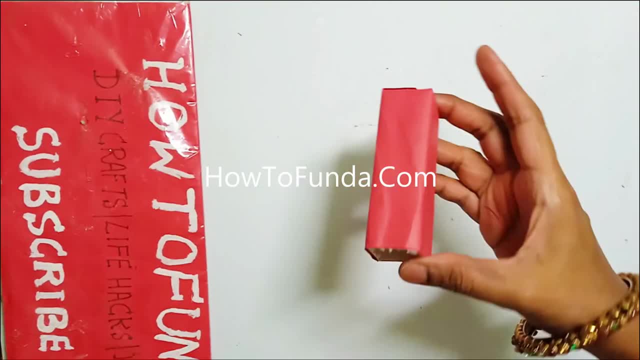 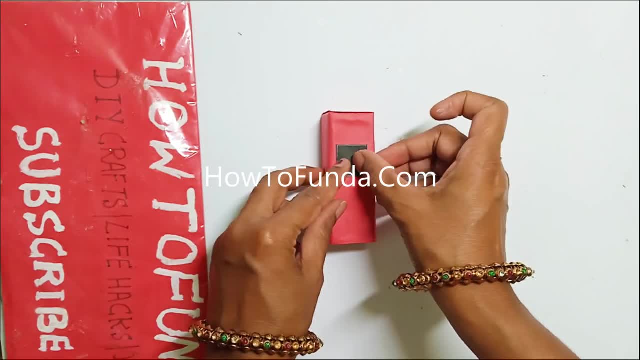 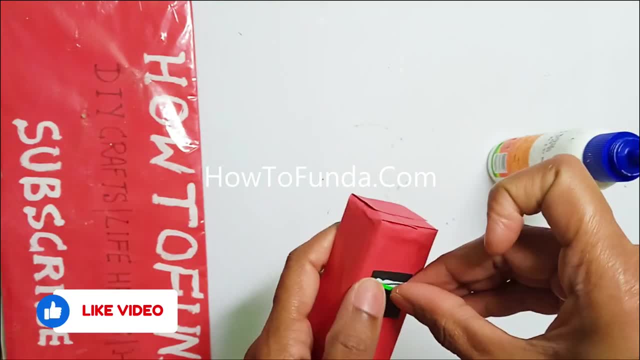 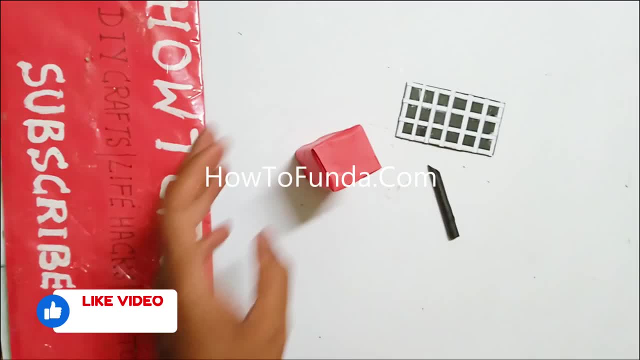 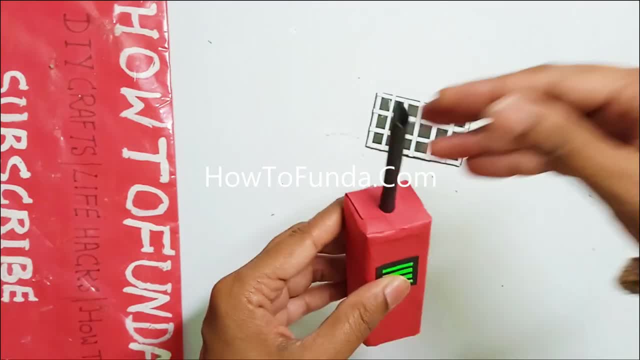 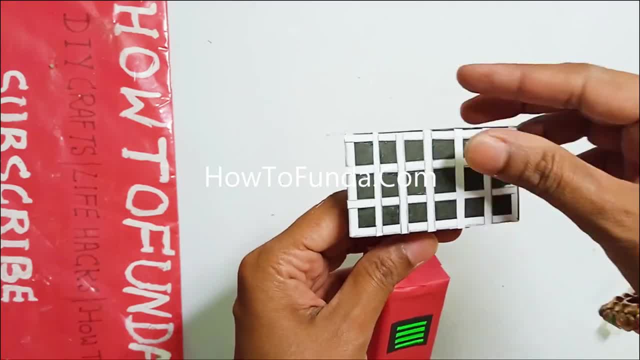 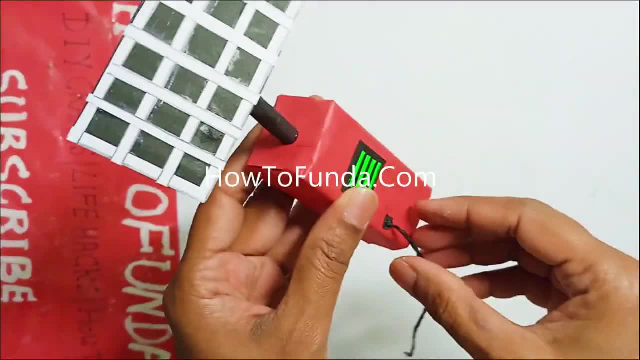 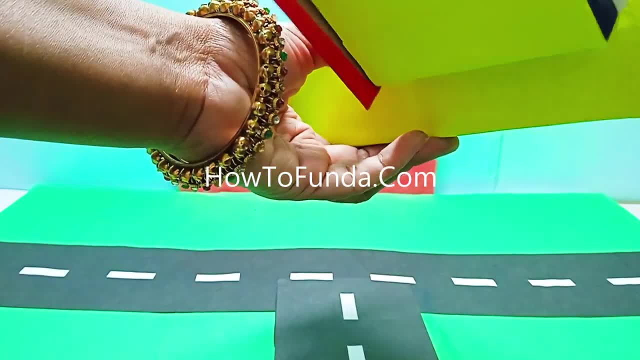 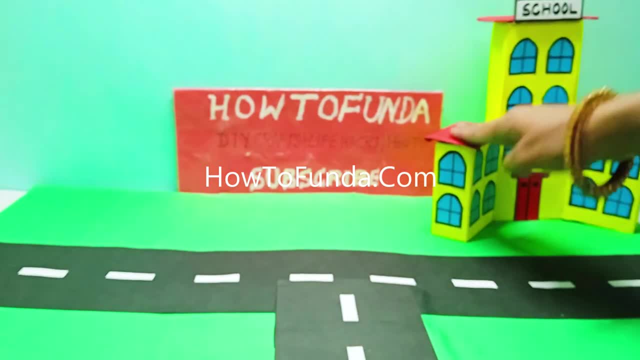 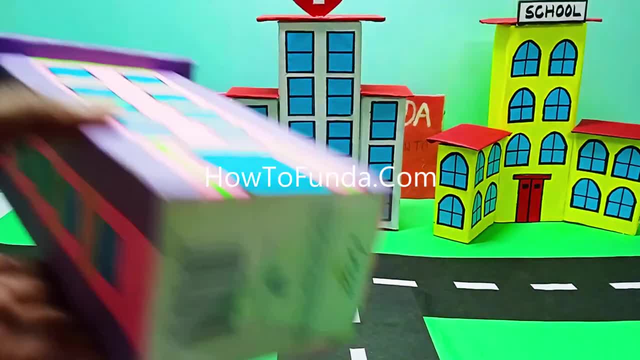 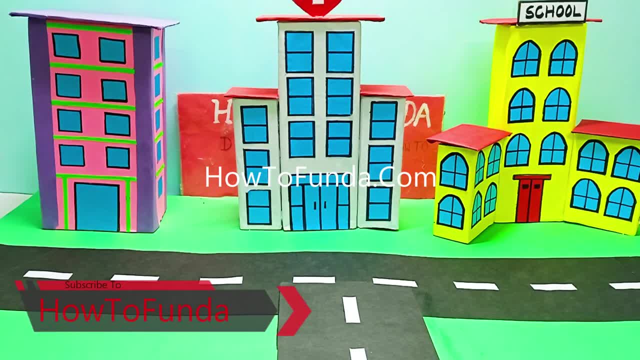 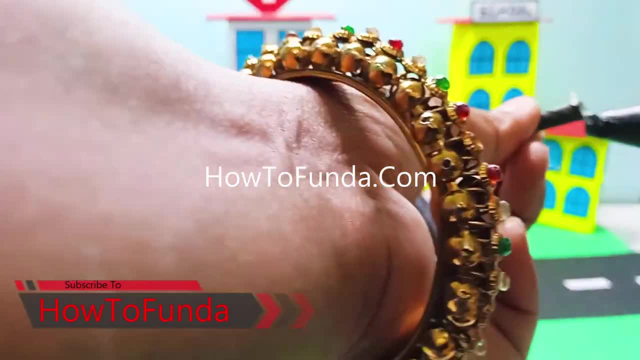 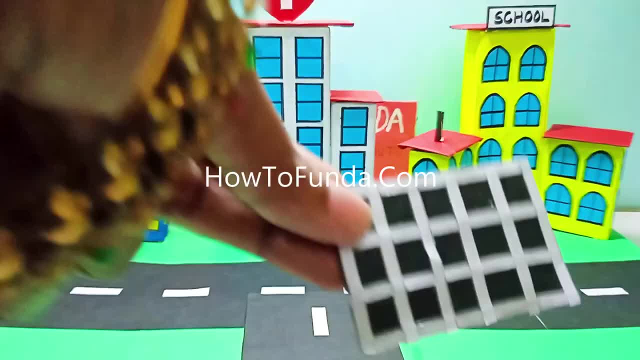 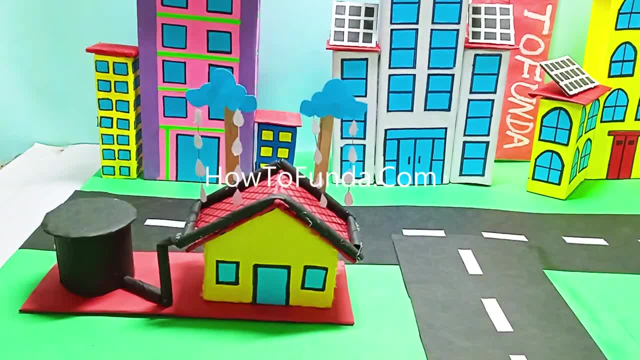 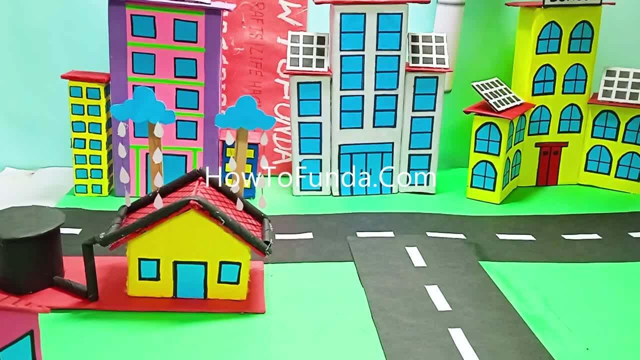 I believe she's so bad that she made the bread. I believe she's so bad that she made the bread. I just do. that's fact and I don't feel no shame. It's a mood you lack. I go crazy, Nah, but I ain't lazy.